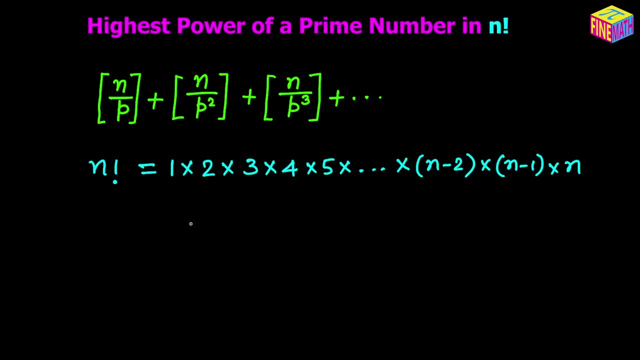 times 5, all the way up to that integer, right. So it's the continued product of all the integers between 1 and that number. For example, if we take a number 15, and what would be the factorial of 15? Well, factorial of 15 is going to look like this. So let me write it down like this: 15 factorial. 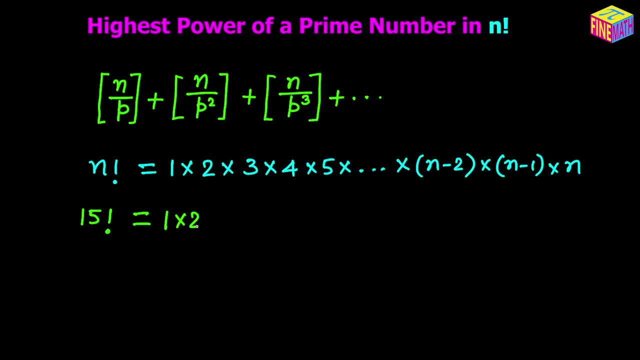 15, factorial would be the product of 1 times 2 times 3 times, 4 times, 5 times, 6 times, 7 times, 8 times, 9 times, 10 times, 11 times, 12 times 13.. Times 14 and times 15.. So this product, whatever is the result of this product, this product will be. 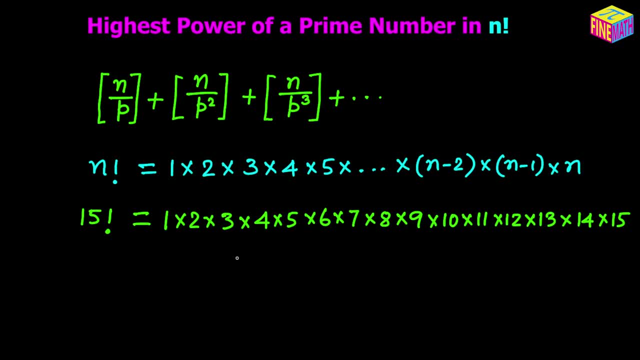 equal to factorial 15.. 15 factorial Factorial of 15.. So factorial is a function that indicates that it is a continued product of all the integers between 1 and that number. And obviously we cannot take factorial of fraction, We need to take factorial of positive integers And also. 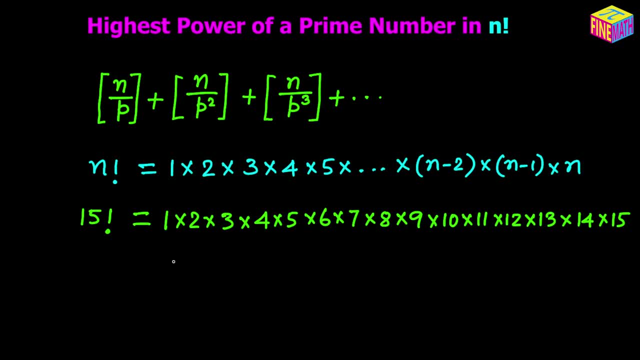 0 factorial is also possible. 0 factorial is actually equal to 1. So any non-negative integer can have a factorial value. So in this example let's play with the factorial 15.. And say, for example: we want to find out the highest power of 2 as a prime number. So we are going to take 2. 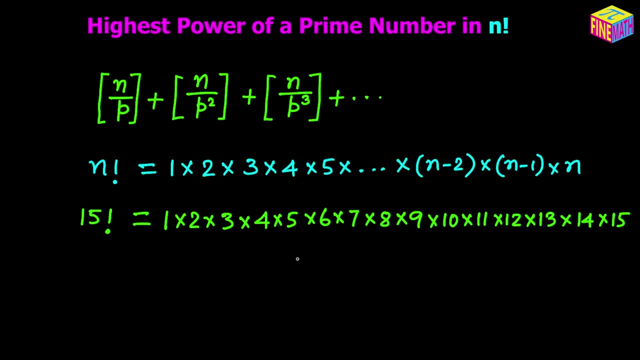 as an example. In fact we could have done it for 3 or 5 or 7.. But for demonstration let's go with the prime number 2.. So from this factorial we are going to try and find out what is the highest power. 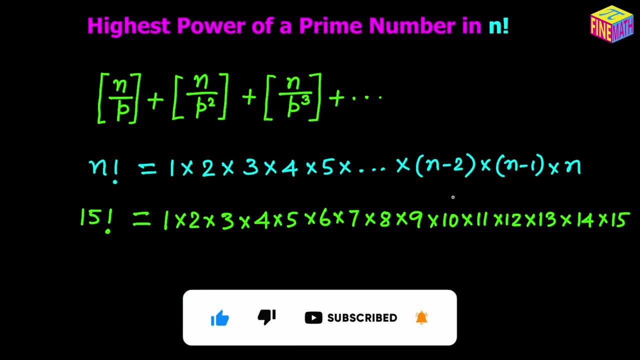 of 2 in this particular value. It's a big number. Obviously it's going to be really big number And we want to find out what is the highest power of 2 in this particular value. So we are going to take the highest power of 2 in this number. You know, if we have to do prime factorization, then what? 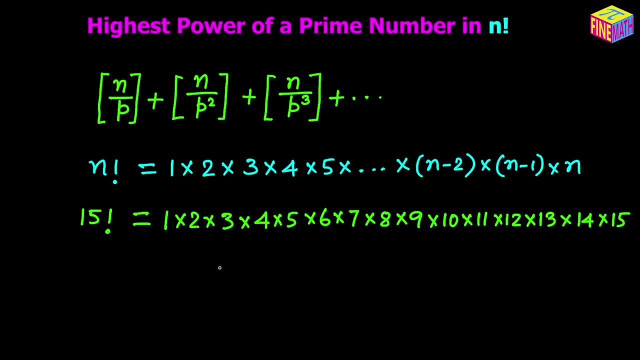 will be the power of 2 in this big number. Well, we can clearly see that we have one of the 2s right here, So this will be one of the 2s. Then here are two more 2s. Then again, here is one more 2. right? 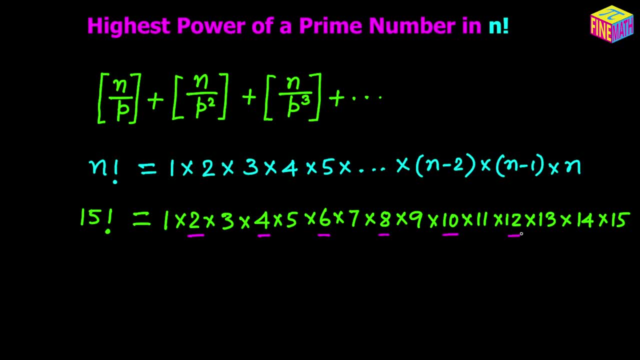 here, Then again three more 2s right here, One more 2 right here, Then two more 2s right there, And then one more 2 right there. So we can sum up all of those to find the highest power of this. 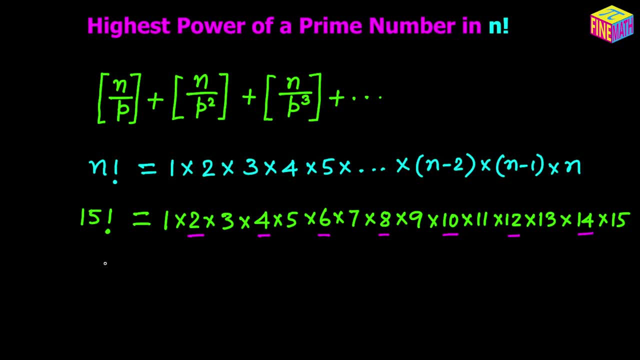 prime number 2 in the 15 factorial Right, Because it's 15. we can easily, you know, write it like this on a piece of paper and find out, okay, what would be the highest power of 2.. But if you are given a really large number, say for example, 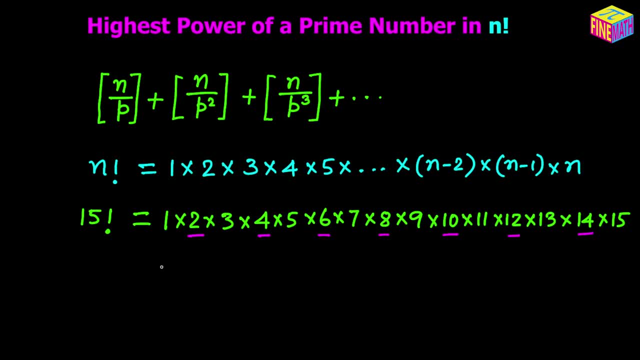 factorial of 100 or maybe factorial of 1000 or factorial of 5000. And you have been asked to find out what would be the highest power of the prime number 2 in that factorial. It will be very difficult to figure it out by writing it on a piece of paper like this, And then you know somehow. 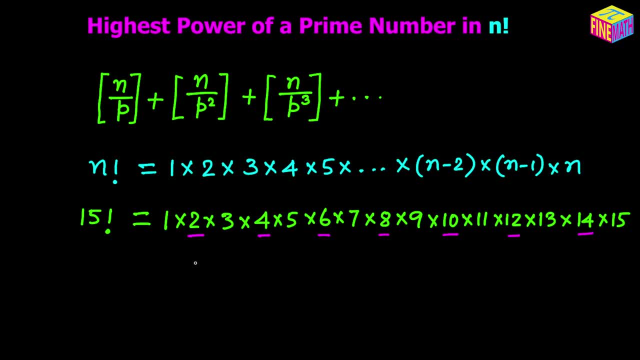 finding out what are the factors of 2 we have. So we have to come up with some sort of a process to find out what will be the highest power of a prime number in a certain factorial. And actually there is a formula. I have written that at the top of. 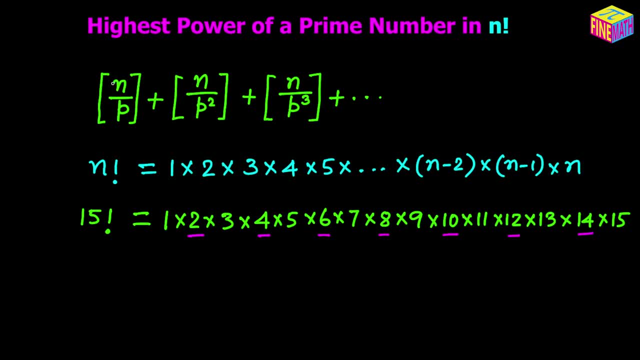 this screen. right here You can see that it would be the greatest integer of n divided by p, plus greatest integer of n divided by p squared, plus greatest integer of n divided by p cubed, and so on until this greatest integer value becomes 0.. So we need to use this formula to find out what is. 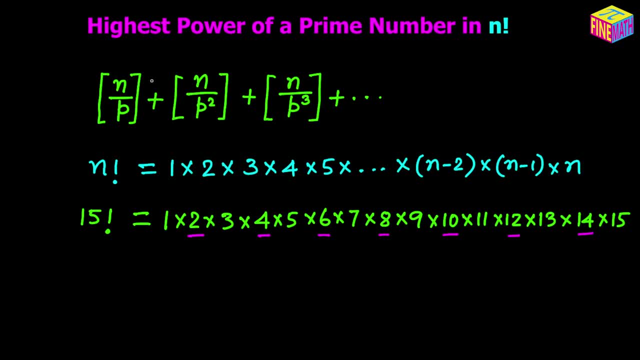 the highest power of this prime number, p, in n factorial. Now the question is, where did this formula even come from? And that's what we are going to prove in this video. So now let's start our game. We have 15 factorial, So we are going to take n as 15.. So 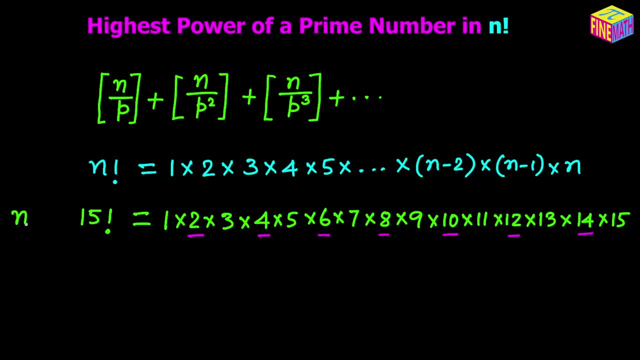 here we are assuming that 15 is actually our n factorial. Our n factorial is actually 15 factorial, So we are taking n as 15, just for demonstration, And then we are going to find out the highest power of 2 as a prime number. So in this case we are taking 2 as our p And. 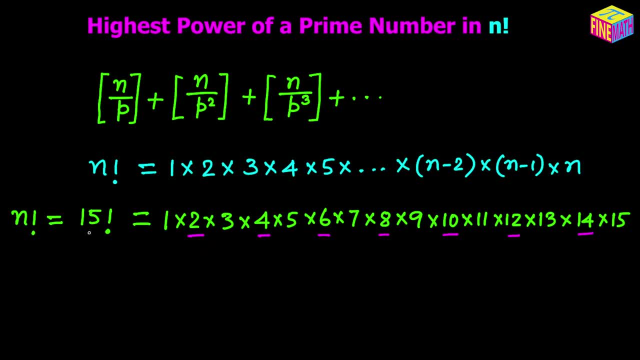 so 2 is the p and n is 15.. So 15 is the n and 2 is the p. With that assumption, we are going to try and prove this particular formula right. So let's get started then Now, before we go too far. one: 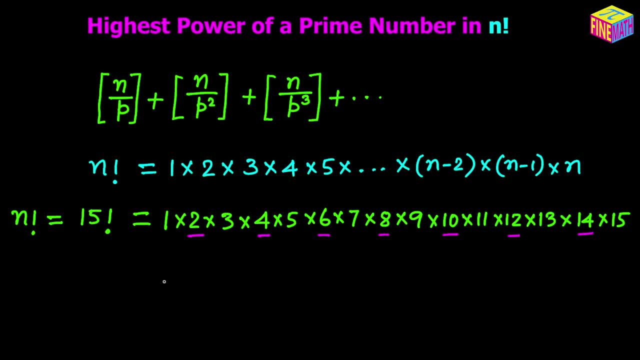 other important aspect we have to understand is: you know, say, suppose, between 1 and 15, how many multiples of 2s are there, Meaning how many even numbers are there? Or I should not say even number, because I have already underlined So it is 1, 2, 3, 4, 5, 6 and 7.. So looks like there are 7. 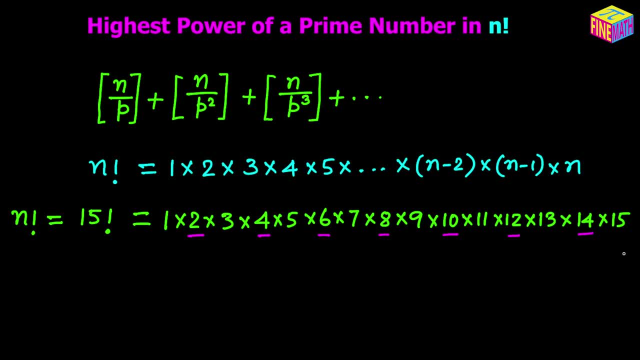 multiples of 2s between 1 and 15.. Now, where is that 7 number coming from? Well, if you think about it, if we divide 15 by that prime number, that will give us how many multiples of that prime number exist between 1 and 15, right? So now this is what I am going to do, that if I divide our number 15, 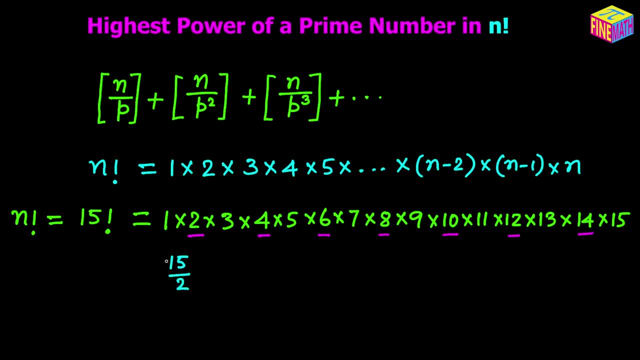 say 15, and I am going to divide that number by 15.. So I am going to divide that number by 15. And this is going to give us the answer 7.. This is actually 7.5.. However, if we take the greatest, 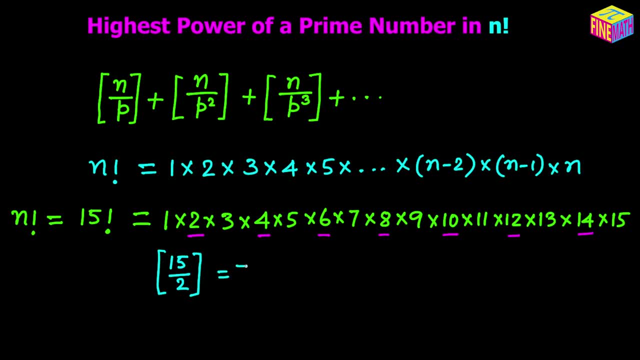 integer of this, we are going to find that this is actually 7.. And you can see the pink underline that I have right here that there are 7 of them. There are 7 multiples of 2 exist in this 15 factorial right. You can see that there are 7 multiples of 2 right. So this is one thing that 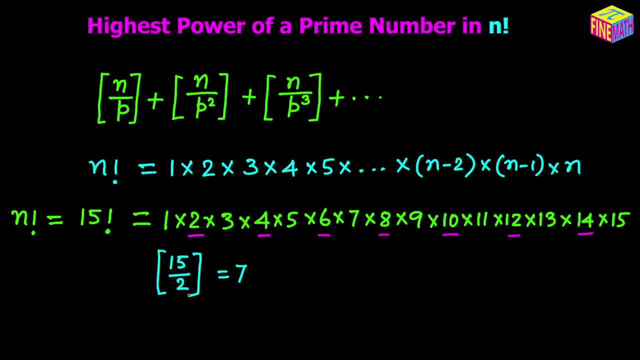 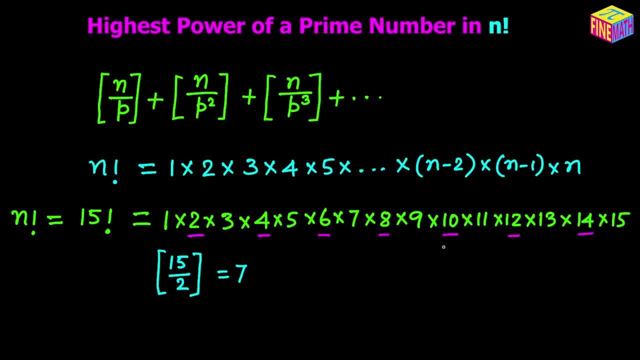 to to figure out how many multiples of 2 would be there. Now also, you should imagine this as n divided by p. That's the first one, n divided by p and the greatest integer of that. That's going to tell us how many multiples of 2s we have in the first round Meaning in this original picture. 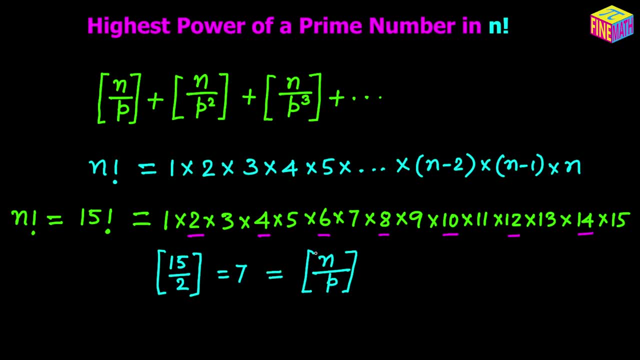 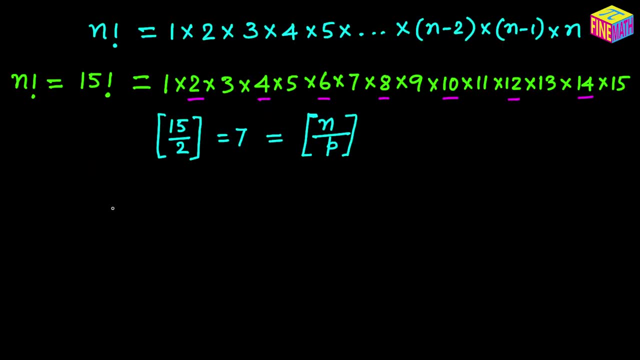 So this is actually equivalent to n divided by p, greatest integer of that right. So now let's get started And as you can see, So in here what we have, I am going to start writing from here. So let's first write down all those multiples of 2s and let's write. 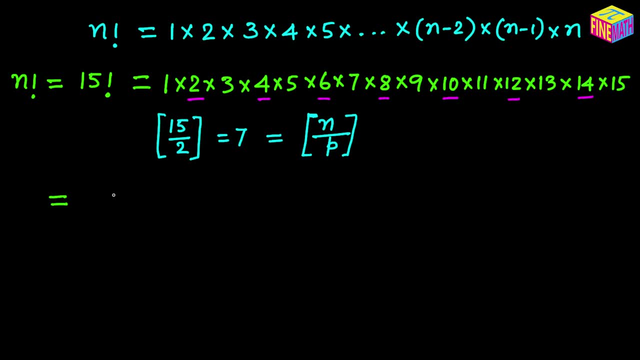 the other terms separately, right? So first I am going to use a parenthesis and I am going to group all the multiples of 2s together. So I am going to write 2 times 4 times, 6 times, 8 times, 10 times 12. 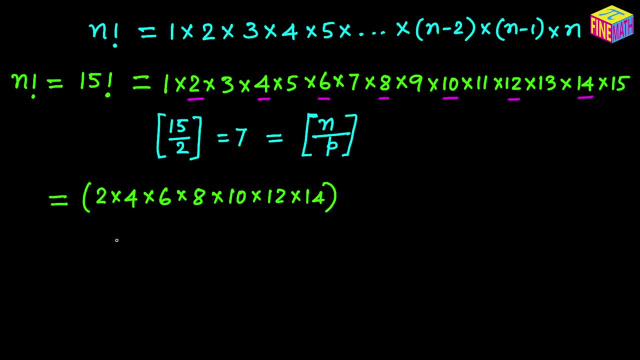 times 14, right? So I am going to group them together because I am interested about those factors only, Because that is where I have the prime number 2.. In all other factors the 2 does not really exist, If you think about 1 or 3 or 5 or 7 or 9.. They really do not have. 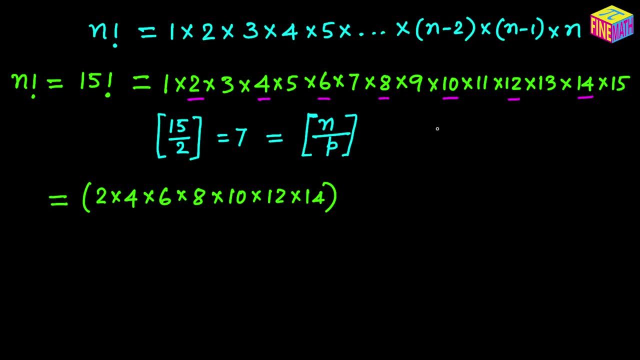 a factor of 2.. They really don't have 2 inside them, So I am not interested about them. So what I am going to do, I am going to write all the multiples of 2s like this, And then times whatever. 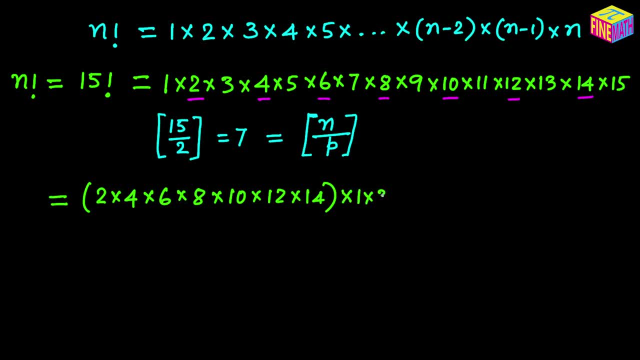 is remaining. Well, what is remaining? We have 1., Then we have 3.. Then we have 5.. We have 7.. It is our factorial 15.. I just rearrange little bit and I am writing it like this right Now from: 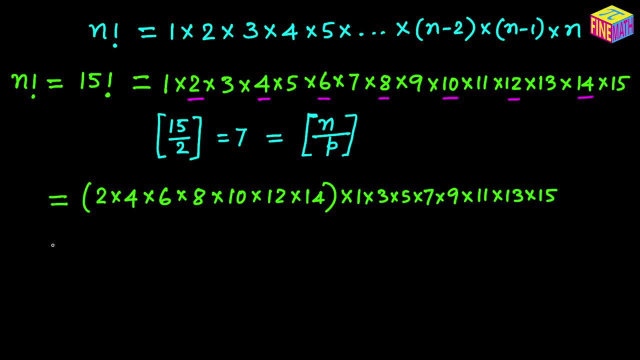 here. you see that. can we write it like this? Can we write it as you know? I am going to write it as Now, how many multiples of 2s we have here? we have 1, 2, 3, 4, 5, 6, 7.. So if you take 2 out from each of, 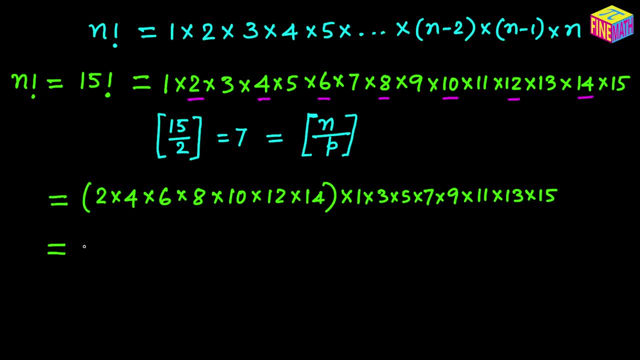 these factors. So if you take 2 from each of these factors, Then how many 2s we will get? We will get 2 to the power 7. We have, we will get 7 of them, and everything is in multiplication form, right. So? 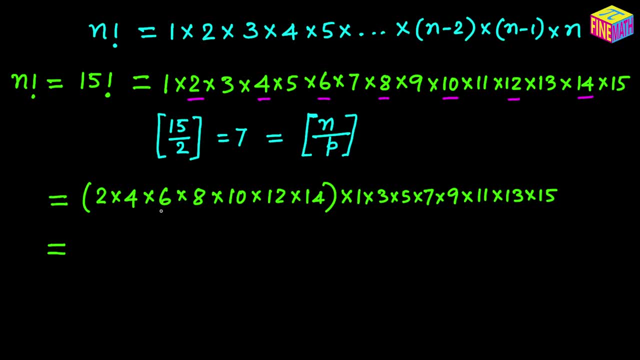 from the first factor, I get a 2.. From the second factor, I get a 2.. From the third factor, I get a 2.. In the first round I am going to take only the 2s out, If you are thinking that, hey, in the second. 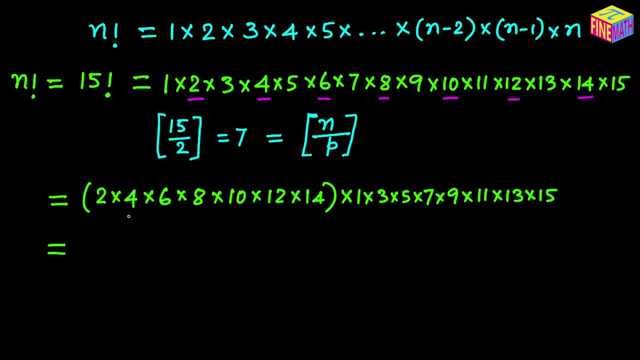 factor. here we also have couple of 2s, But I am going to take only 1- 2 out of each of these factors in the first round. So we have 7 of them here: 2, 4, 6, 8, 10, 12 and 14.. That's 7 multiples of 2s And I. 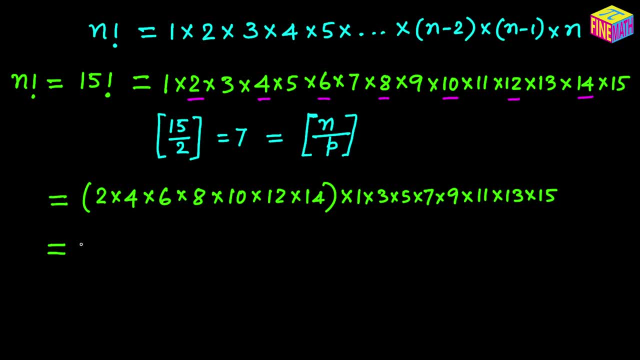 am going to take the 2 out of each of the 7 factors there. So I am going to get 2 to the power 7.. That's 7 of the 2s I get. And then, within parenthesis, what is left? Well, from the first factor, we will. 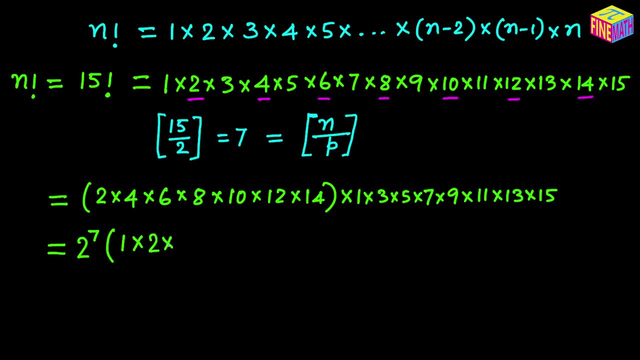 have: 1. From the second factor, we will have 2.. From the third factor, we will have 3.. Then from the fourth one, we will have 4.. Then from the fifth one, we will have 5.. Then from the sixth one, we will. 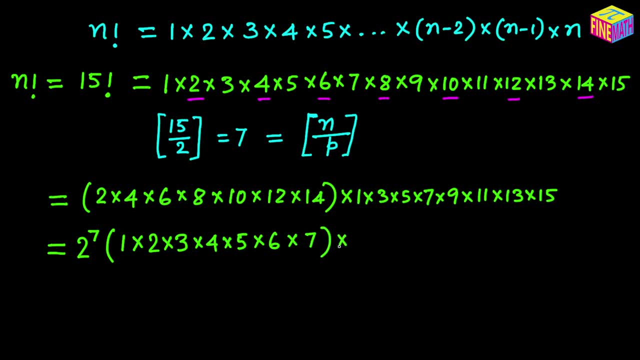 have 6. And from the seventh one we will have 7., And then outside, whatever we have this number right here, I really don't care about this portion right here. This is just an integer. It is some integer And I am really not interested about that integer because it does not contain a factor 2.. So 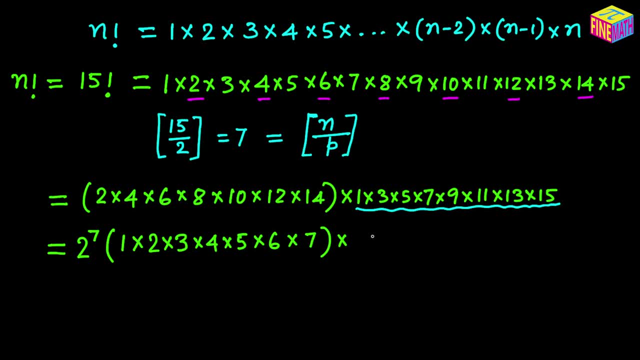 I am really not interested, right? So what I am going to do, I am going to write it as some some integer a, Let me just say like a lowercase, a right. So that's just some integer a, And I am not really interested about that, Because I am interested about only the factors. that contains 2.. 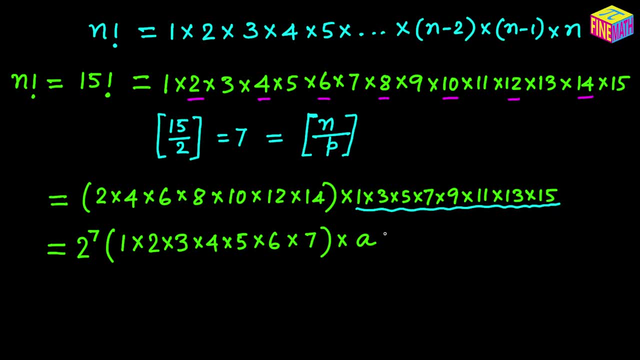 But those other factors don't contain 2.. So I am just simply replacing them with some integer, a right. So now, from here you see, okay, So we have 2 to the power, 7 times this right. Now you think about these remaining factors within the 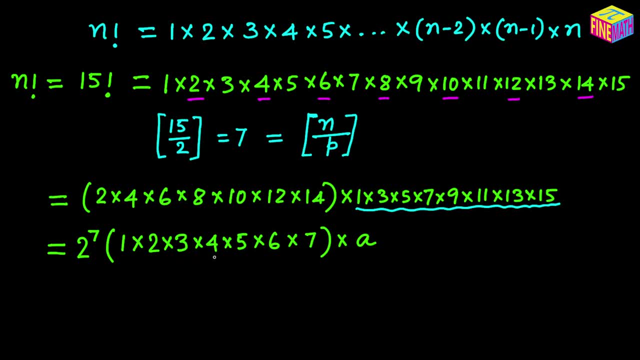 parenthesis, Now, how many factors we have? Well, we have 1, 2, 3, 4, 5, 6, 7.. And out of those, how many multiples of twos we have? We have 1, 2 and 3. We have three of them. And how did I get this number? 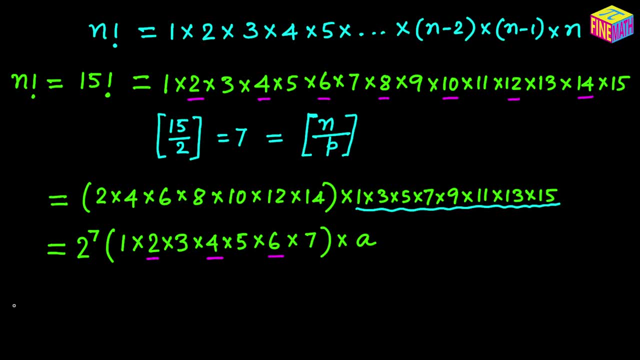 3. Well, this 3 is actually. if you think about it, This is nothing but 7.. So if you say 7 divided by 2. And you take the greatest integer of that, That's going to give you 3.. So now we know that. 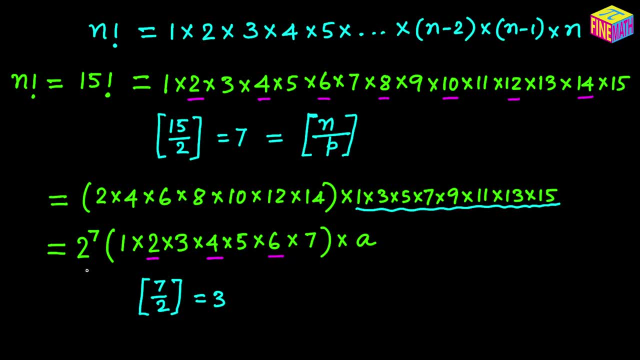 we clearly have three multiples of twos inside there. all right, Now, if that is the case, I am going to erase this And let me say okay. So now I am going to rewrite this thing as 2 to the power 7.. And then, within parenthesis, I am going to keep only the multiples of twos, Like 2 times 4 times. 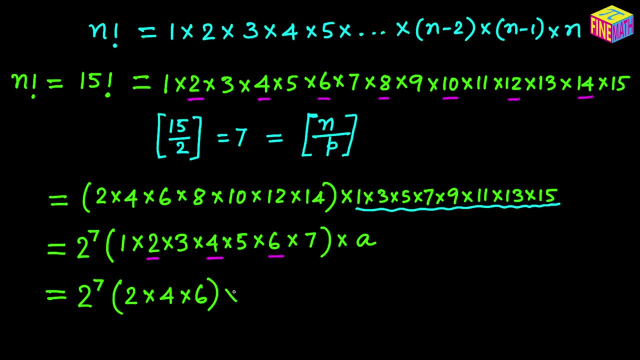 6, right, And then I am going to bring everything else outside, Outside. I already had another integer a And then I am going to bring this 1, 3, 5 and 7 outside, So 1 times 3 times 5 times 7.. So I am going to bring all of them outside of the parenthesis And then 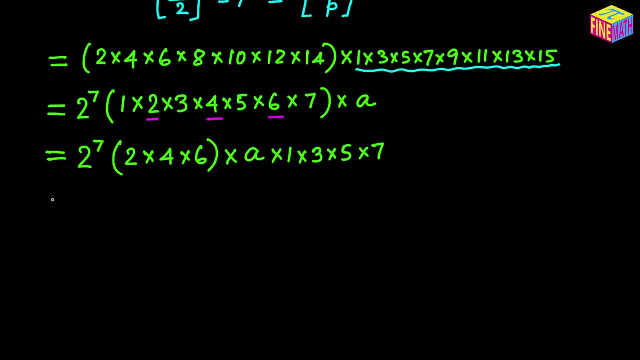 from within the parenthesis what I am going to do. I am going to again bring out as many twos as I can. So how many twos I have? Well, I have 1, 2 and 3.. I have total three twos there, right? 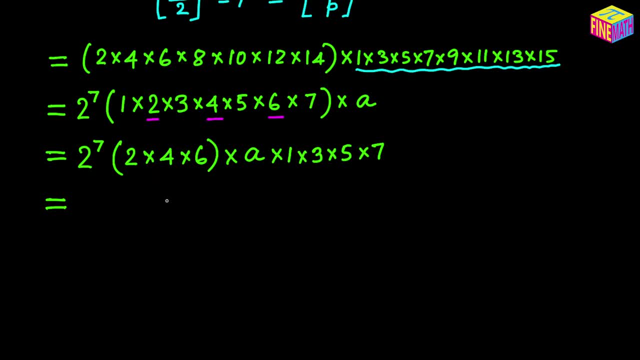 I know that there is one more two in the four, But we will do that in the next round, So in in this round I am going to bring out only the three twos out of here. So a two from the first factor And then one more two from the second factor And one more two from the third factor. 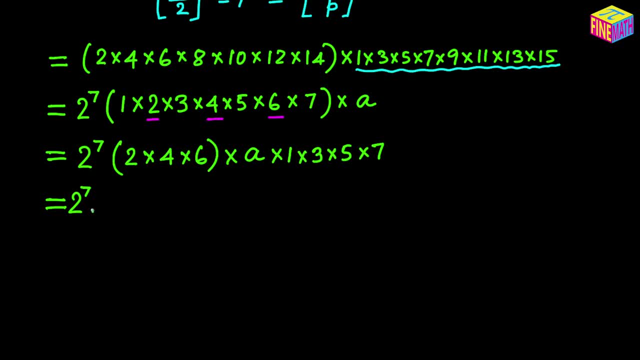 I already had two to the power seven, And then now also, I am getting another two to the power three. And then, within parenthesis, what we are going to be left with? Well, we will be left with a one and a two and a three, And then, times, we have this, a multiplied by a bunch of other integers. 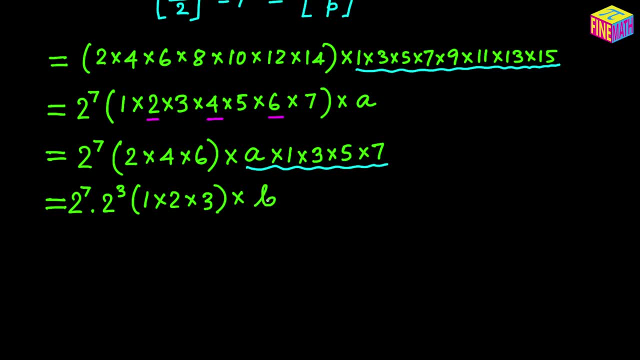 And I am going to call it a, b. You know, I am just, I am really not interested about them. So I am just using symbolic here, right, I am using like algebraic symbol here to indicate that, hey, there are some integer, There is just some integer that I am not interested about. But I we really cannot. 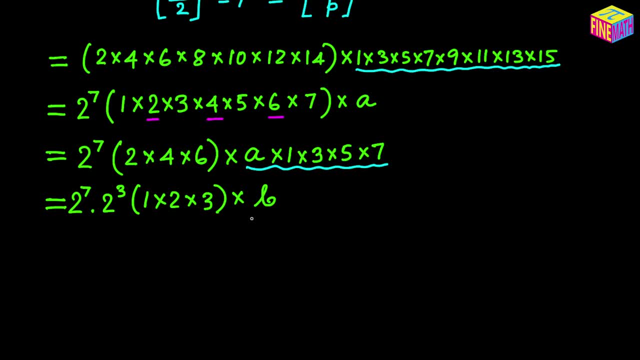 ignore it, So I am keeping it. But again, it does not do anything for our purpose, right? So I am just keeping it like that. So now, you see, now we are at a place where we can, we can write it like this, So we can say: okay, this is nothing but two to the power seven plus three, We can add the. 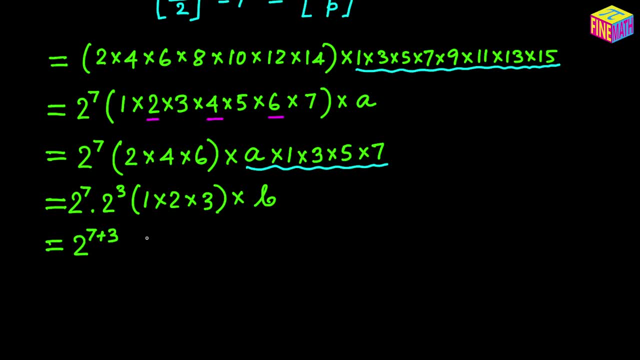 exponents, because everything is in multiplication form. And then, from within the parenthesis, again, what I am going to do: I am going to keep only the multiples of twos. Now, how many multiples of twos we have. We have actually one. Now, where did I get that value one? Well, if you think about it, we have. 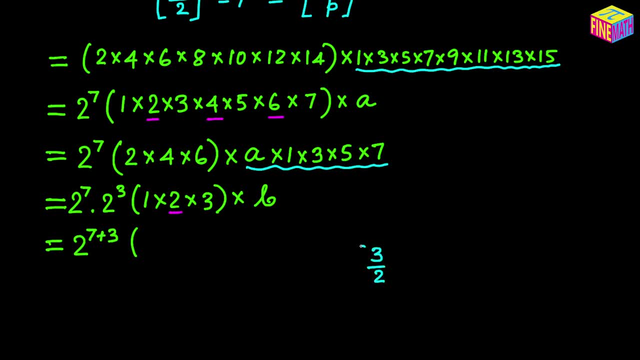 three factors. And if you say three divided by two, Take the greatest integer of that, What are you going to get? We are going to get one. That means between one and three. we have only one multiple of two right. So if we keep only the multiple of two within the parenthesis, then it is going to look 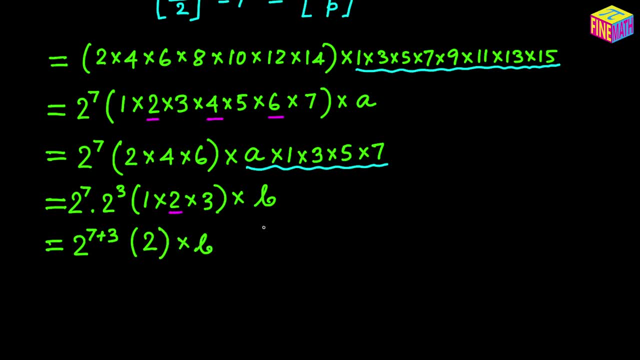 like this, And then we already have the b right here, And then I am going to bring the one and the three outside, So I can say: times one, times three, And we are going to write it like this. So now we are going to say: okay, It is now going to be two to the power, seven plus three. We are going to 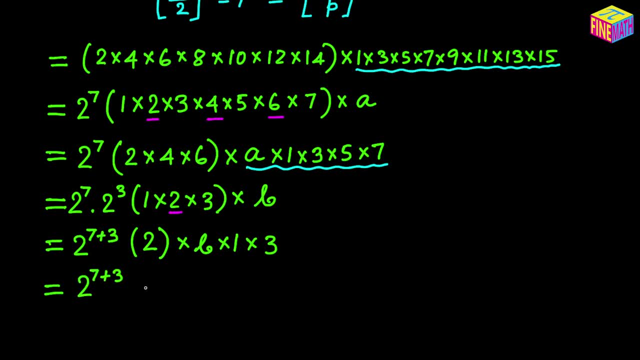 say two to the power seven plus three, And then, from within the parenthesis, you see I can bring out one more two. right, Because there is only one factor of two, And I can bring out one more two. So let me say, okay, this times two. And then, within the parenthesis, we are going to be left with a one. 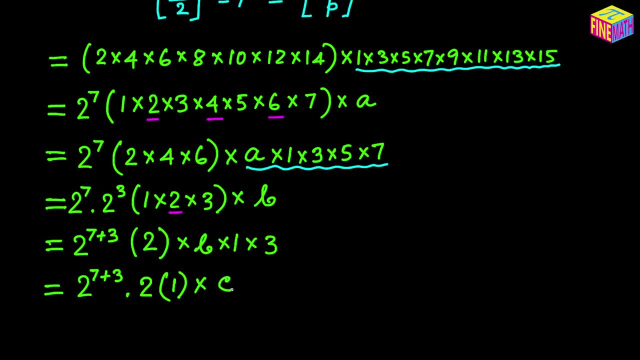 And then times b, times one times three, Let's say this is nothing, This is like a, c, So from where you can say: okay, So this is looking like two to the power seven plus three plus one, Because we can write it as c, So I am adding the exponents there. So two to the power seven plus three plus 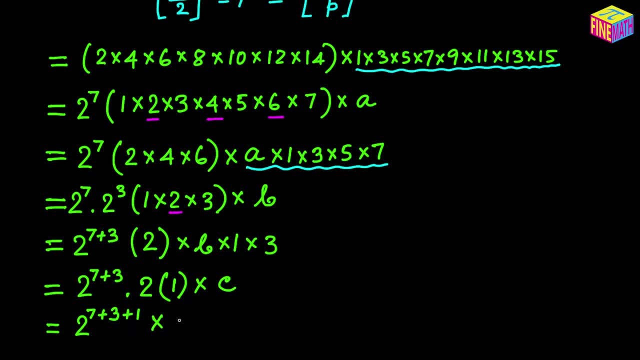 one And then times. we have one times c, So we can write it as c. So finally, you see that we have been able to find out what is the power of our prime number. So the power of our prime number in factorial 15 is actually this sum right here. This is what we are interested about: The seven. 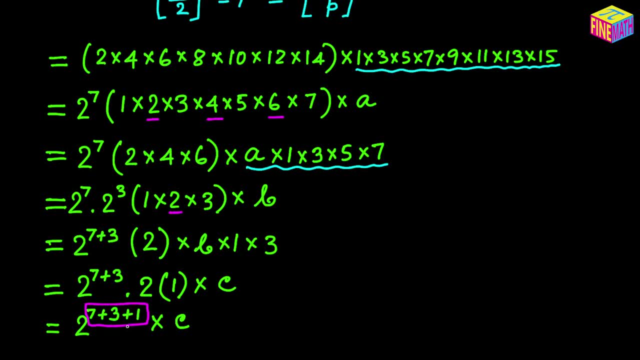 plus three plus one. That is what we are interested about- That there are actually eleven twos hiding in factorial 15.. That means the highest power of two in factorial 15 is going to be seven plus three plus one, which is equal to eleven. Now if we try that in the formula, The formula that we had, If 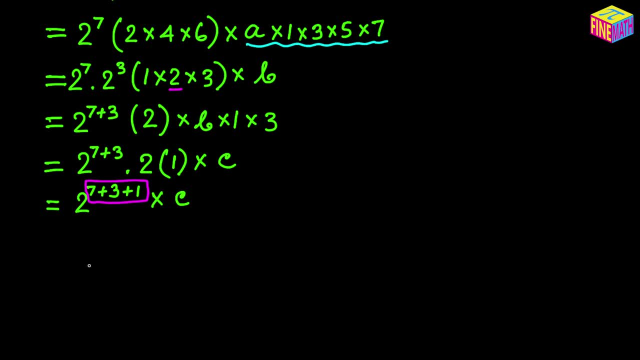 we try it in our formula there. So the formula that we had, We had the formula like this: n divided by p, greatest integer. plus again n divided by p, squared, greatest integer, plus n divided by p, cubed, greatest integer, and so on. So here, if we use: 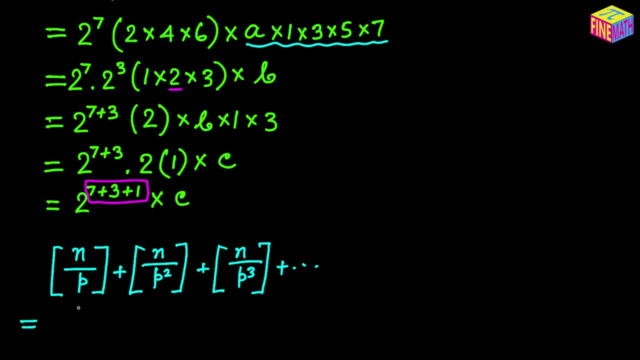 n. So what do we get? Well, it will be greatest integer of fifteen divided by two. Two is our prime number in this example, So it will be like this: Then it will be fifteen divided by two squared, Which is four, Two squared, That is p squared, Which is two squared, And then again fifteen. 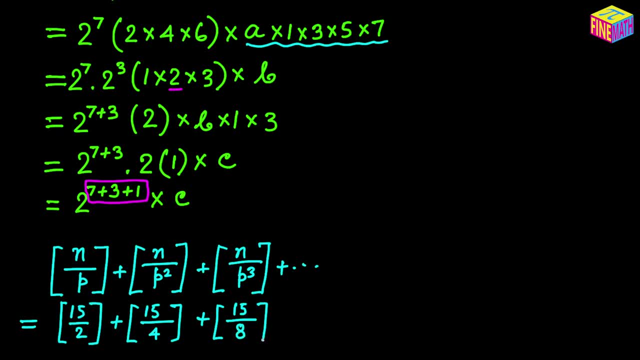 divided by two cubed, That is eight. And then do we need to continue anymore? No, Why? Because then the next item would be fifteen. divided by t to the power four, Which is two, to the power three, the power 4, that would be 16. and guess what this greatest integer will come out to be 0, this one. 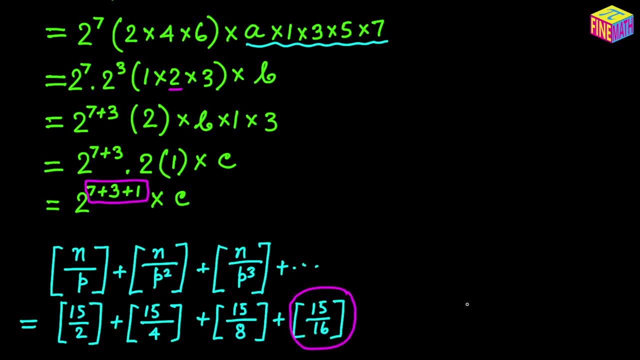 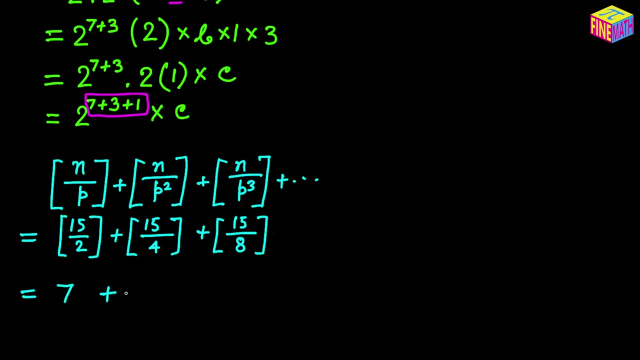 will become 0, so we really don't need to continue anymore. so we can pretty much stay with the three terms here and now. let's see, uh, what we get. so from here we are going to get 15 divided by 2, that is 7.5. greatest integer would be 7 plus 15 divided by 4, that would be 3, point something. 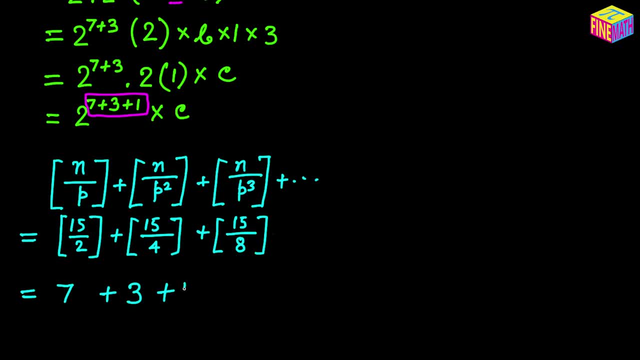 greatest integer would be 3 plus 15. divided by 8, that would be 1 point something, so the greatest integer will be 1, so this is equal to 11, and that is the highest power of our prime number 2 in factorial 15.. now, so far, we have been able to validate that. yes, the formula is actually working. 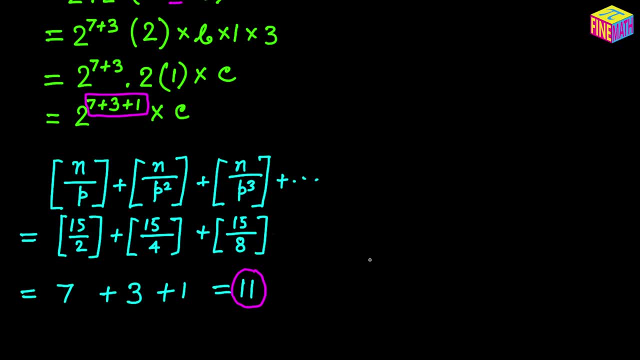 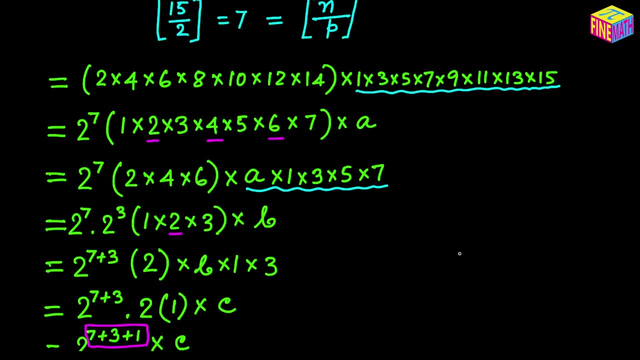 based on what we noticed. right now, i am going to show you where the formula even came from. actually, the formula came from this derivation only. so if you look at this derivation, we should be able to figure out how many twos we are getting. now, here you see the two to the power seven that. 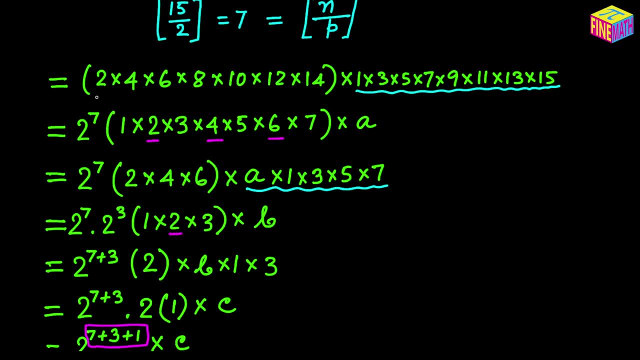 we have right here that two to the power seven is nothing, but the number of multiple of two is between one and fifteen. right, so that is that seven. right here we can say: okay, this seven, this seven, is nothing but n divided by p, the greatest integer function of that, that is. 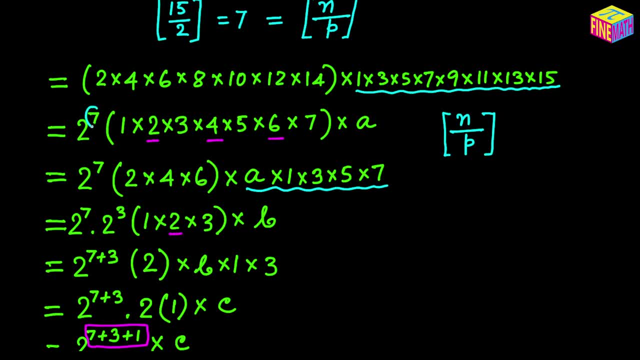 actually the seven, so in our case the seven that we got right here. two to the power. seven, that is nothing but n divided by p. it's just how many multiples of twos we had between one and fifteen right, that is that seven, and then the other three that we got well. 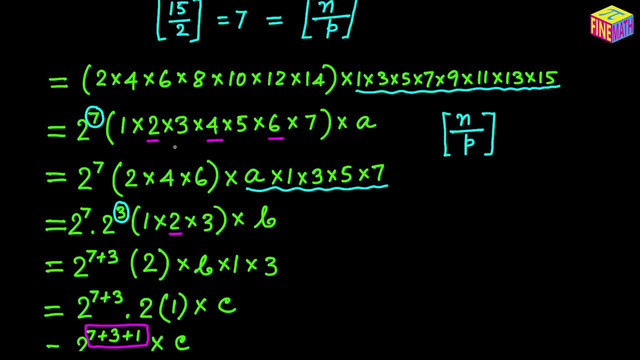 if you think about it. so, once we are done with that, how many terms did we have here in here? if you look at this particular portion right here, now i am going to use a different color. i am going to use the white color. if you look at this portion right here, how many terms we have? well, we have. 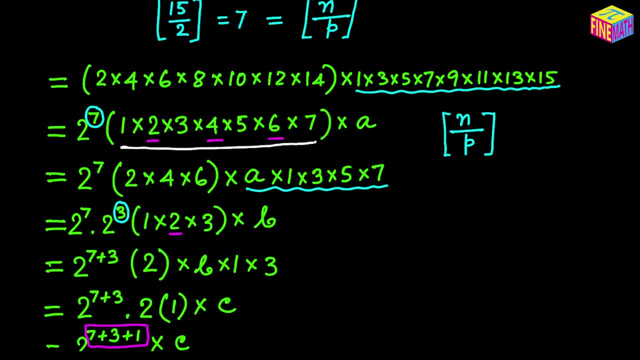 n divided by p. greatest integer of n divided by p. we have so many terms here now, from there again. so if we have greatest, if we have so many terms in there- in this case it is actually seven terms there- but we can use the symbol x and we can. 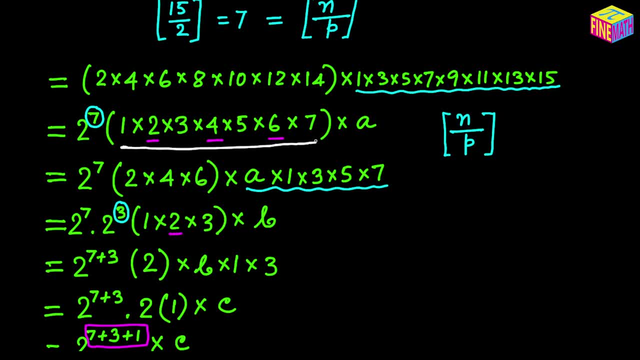 say: okay, we have actually greatest integer of n divided by p. so many terms we have there now in that many terms, how many multiples of twos we have. well, the number of multiple of two would be again, whatever that is, you know, the n divided by p, n divided by p, and then i have to divide that. 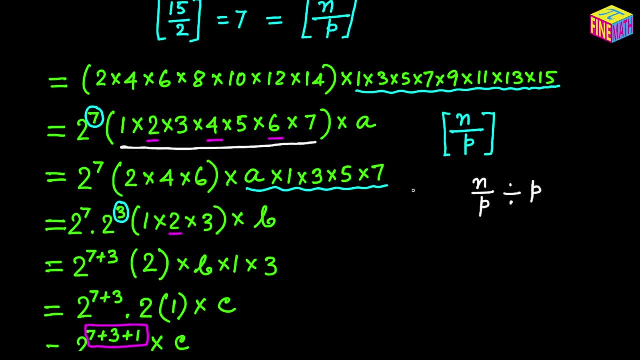 by p again, because we are trying to find out how many terms we are going to get in this- other parenthesis right here- how many multiples of twos we are going to get. well, we are going to get so many multiple of twos like, like this: the greatest integer function of this, and this is actually nothing but n- divided by: 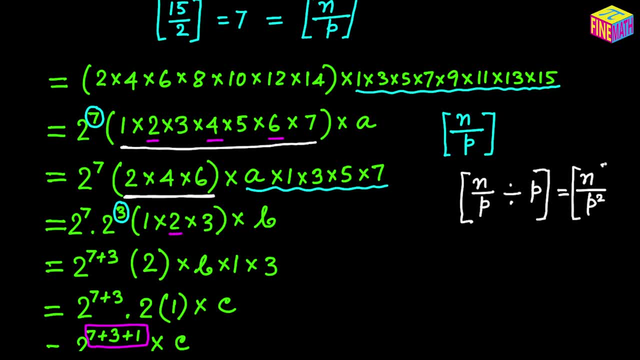 p squared. if you carefully look at it, this is nothing but greatest integer of n divided by p squared. so this is saying that, hey, in the second round you are going to get only so many multiples of twos. in the first round you had these many multiples of twos, and then in the second round, 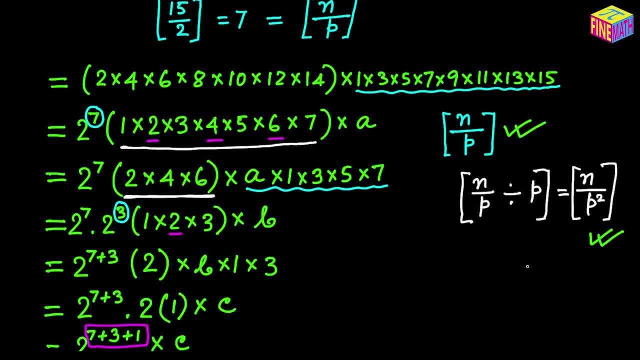 you get so many multiples of twos, all right, very good. now in the third round, how many multiples of twos we get? well, i am again underlying with a with a white color line here. So you can see that in the third round we are going to get how many multiples of twos? Well, the formula would be again: how? 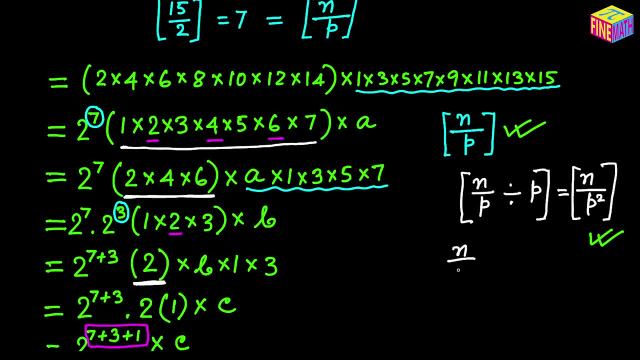 many ever we had before. So before we had n divided by P square, we had so many, and again I have to divide that by P to figure out how many multiples of twos that we are going to get. And this is actually nothing but n divided by P. 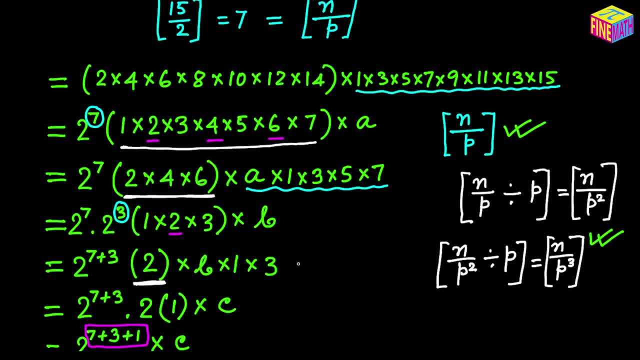 cubed and greatest integer function of that right. So in the third round, how many multiples of twos we are going to get? Well, that's actually n divided by P cubed, because we had n divided by P squared number of terms. and then we 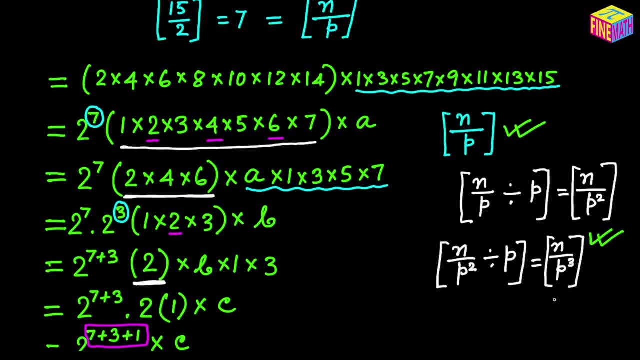 divide that by 2, which is P in this case, and we are going to get so many multiples of twos, and that is why, finally, we get that one of the twos right here, which is right here. I'm going to do a white circle right here, You see. 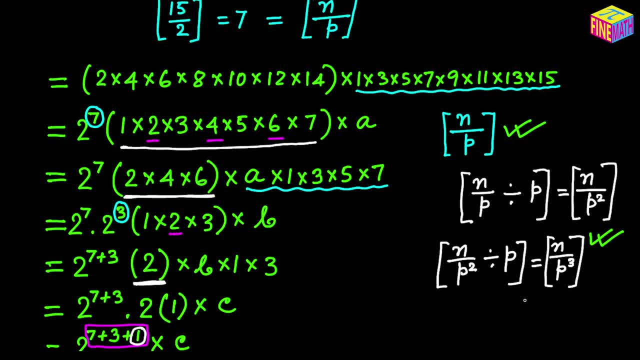 that one of the twos that we got right here, that's actually n divided by P, cubed and the greatest integer of that. So every time you have to understand this, that in, in, at the very beginning, how many multiples of twos we had, We had greatest integer of n divided by P, So many multiples of twos. 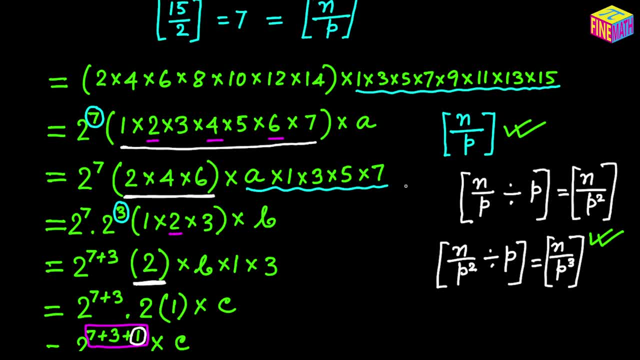 we had Then in the second round, how many multiples of twos we had. We had n divided by P, divided by P again, because we had only so many multiples of twos, and then from so many factors again, how many multiples of twos we get. We get n. 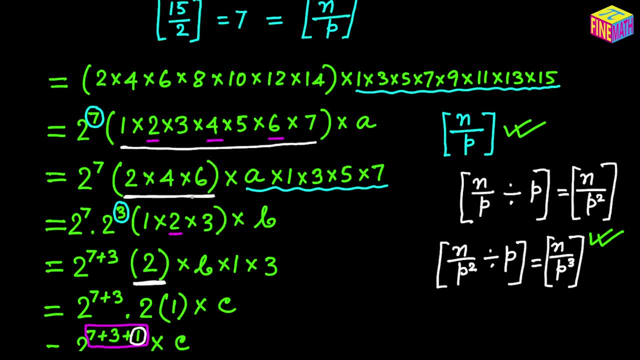 divided by P squared. So many multiples of twos. Now again, once we take out a 2 from each of those factors, then again we are going to be left with n divided by P squared, number of term. and again there are how many multiples of twos we have. We have n divided by P cubed, number of. 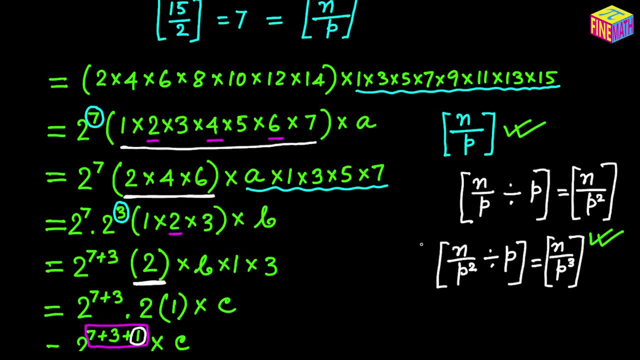 multiples of twos that we have in there. So this is how this iteration will go on until we are done capturing all the factors of our prime number. So from here, ultimately, you see that our 2 to the power, 7 plus 3 plus 1, this is actually. 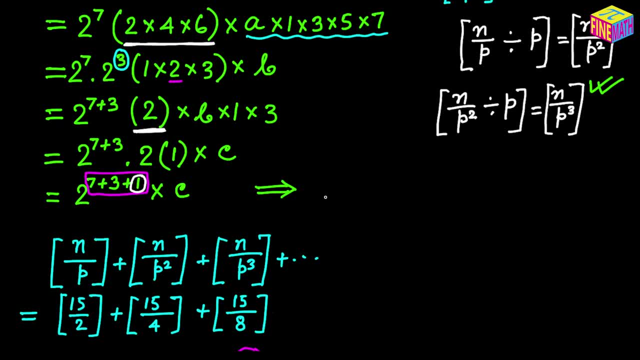 so now I'm going to write this: 2 to the power 7 plus 3 plus 1, that is actually like this, So you can say: okay, we have 2 to the power 7 plus 3 plus 1. that is actually like this, so you can say: okay. 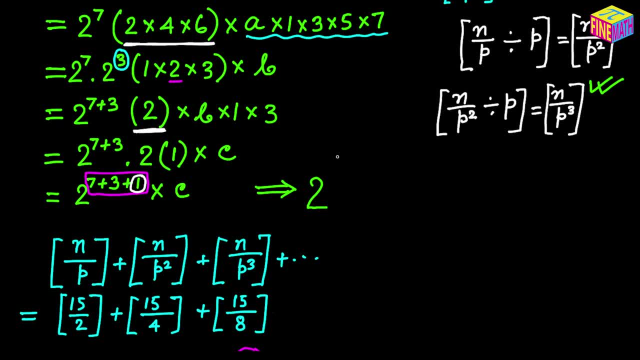 Ok, this is our prime number. Then the first, the 7, is actually 15 divided by 2. greatest integer of that, That is 7. and then the 3 that we have, that is actually 15 divided by 2, squared, which is 4.. I'm going to write it as 2. 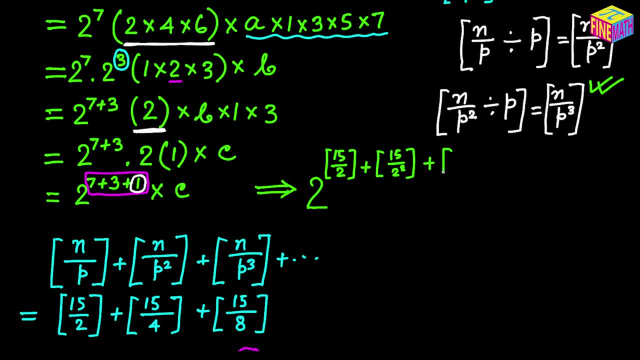 squared greatest integer of that and then the 3 that we have again is actually 15 divided by 2 cubed, which is 8. I'm going to write it as 2 cubed- 15 divided by 2 cubed and the greatest integer of that. So the power of. 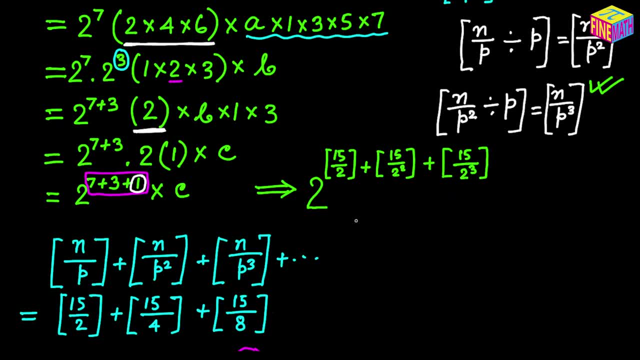 and the greatest integer of that. so that is the power of our prime number 2 that we got from factorial 15. so you can see that how in the first round we got 15 divided by 2, so many multiples of 2s. then in the second round we got 15 divided by 2, squared, so many multiples of 2s. then in the 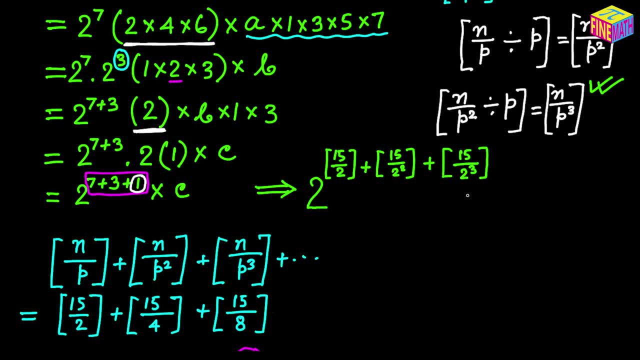 third round we got 15 divided by 2 cubed, so many multiples of 2s. then if we had even more 2s, you know, like a fourth round. yes, we could have continued on to the fourth round if our number was bigger than 15 factorial, and it really doesn't matter how large the number is, meaning how large. 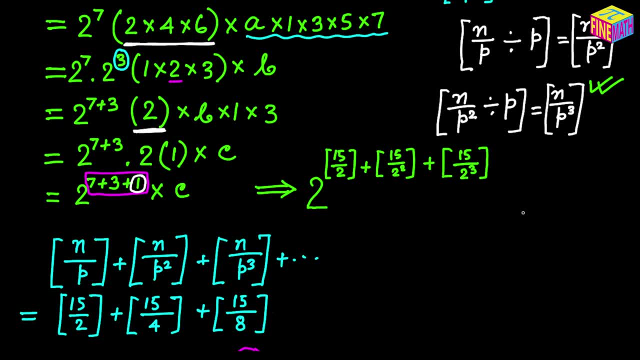 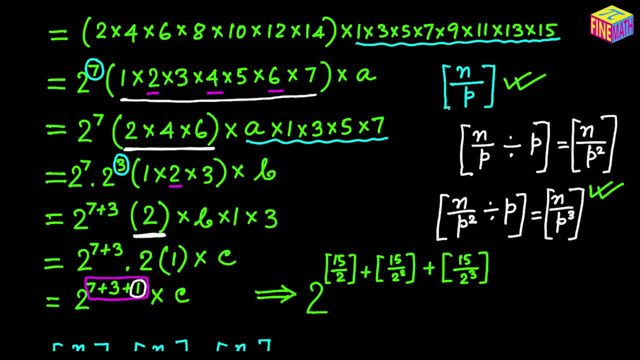 that n is. you can pretty much use this particular formula and you can see how the formula is developing. you know, because in in the first round- again, i repeat, in the first round- we had n divided by p, so many number of multiples of 2s. then in the second round we had n divided by p, squared. 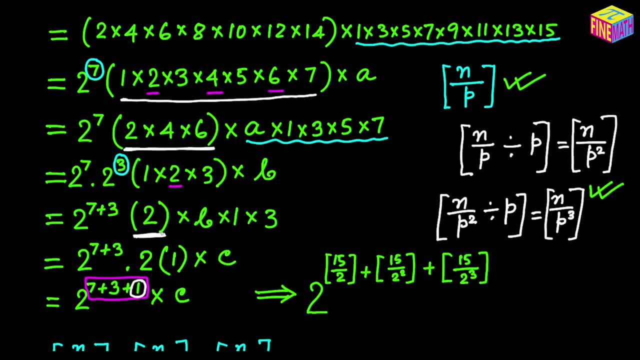 number of multiples of 2s. and in the third round we had n divided by p, cubed number of multiples of 2s, and that is how we are gathering the number of 2s that we have in this large number, which is the factorial 15 right. 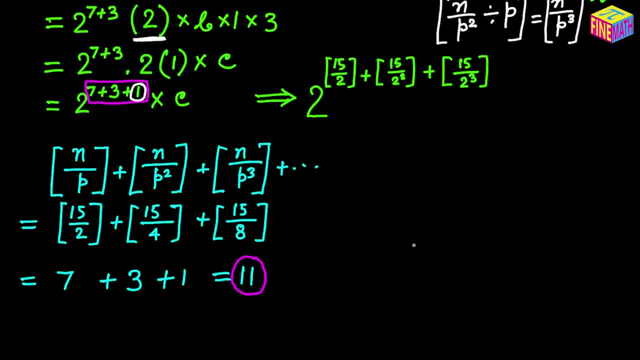 so now, if we replace all of these with n and p, so this particular value right here, let me show you with a, with a pink box right here. so this is the power of our prime number. this is the power of our prime number in factorial 15. so this power, this is the item that we are interested about. so this is. 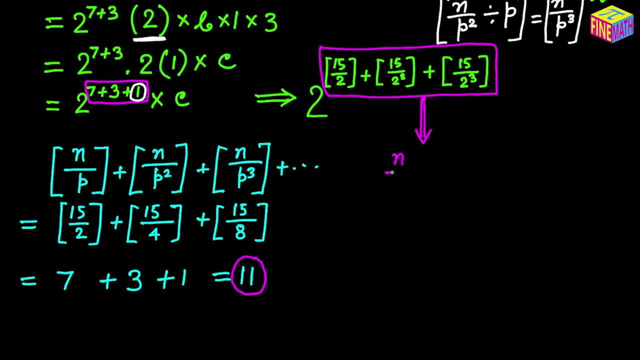 actually nothing, but it is actually n divided by p. that is the first item. i mean, of course, greatest integer of that plus n divided by p squared, greatest integer of that plus greatest integer of n divided by p cubed. so in our example we stopped at p cubed because we only went with number 15 and prime as 2, but it could continue even further. 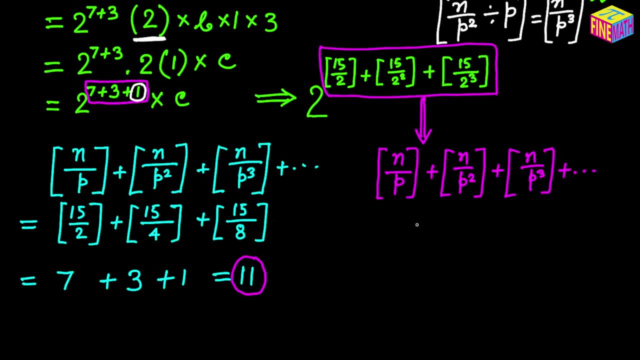 until this greatest integer becomes start to become 0 right. so that is where the formula came from, and this is the formula that says that in factorial n you will have so many p's where p is a prime number right in this factorial n. this is the 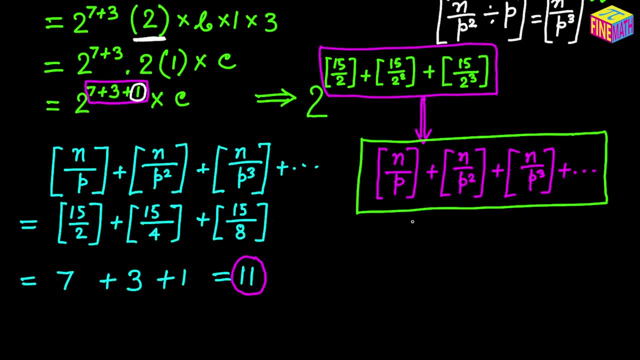 number of p's, meaning the power of the prime number p. so this is actually the power of the prime number. so let me write it down here. this is the power of, or the highest power. you can say power of prime number p in n factorial. so you can say: in where? in n factorial, in n factorial. so this: 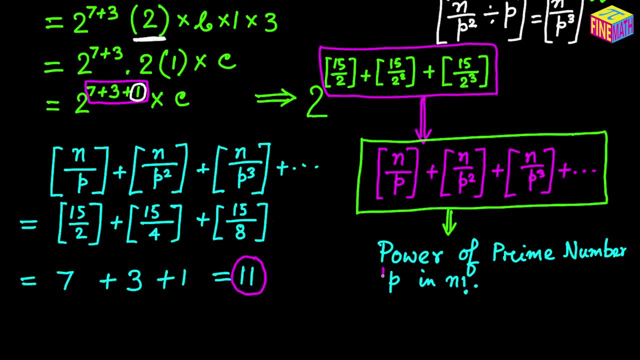 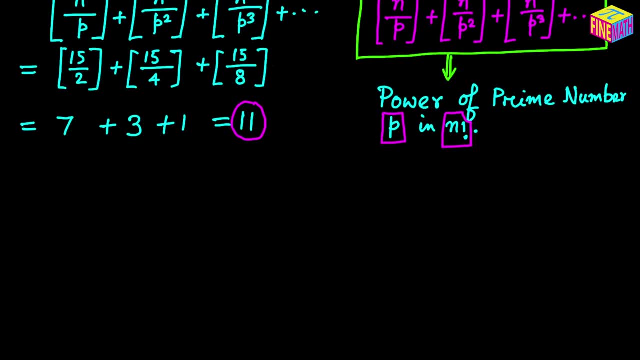 is nothing but the power of the prime number p in n factorial. so this is the power of the prime number. So this is the power of the prime number p in n factorial. Now let's take an example. So suppose you are given that, hey, can you find out what is the highest power of 3 in? 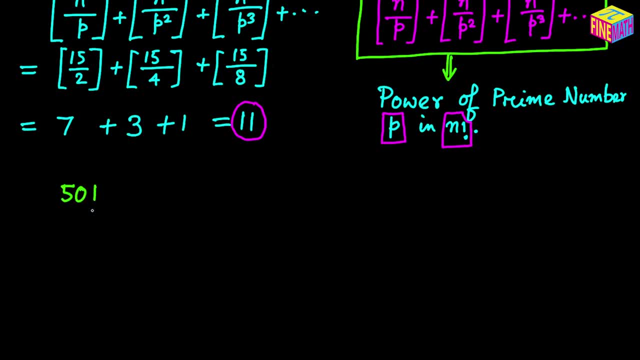 factorial 50?? Sure, we can do that. So we are talking about n as 50 and we are talking about prime number, prime number as 3.. So we have been asked to find out the highest power of 3 in 50 factorial. 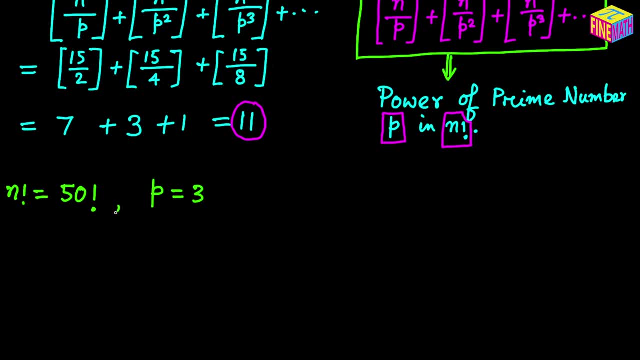 So here n factorial is 50 factorial and our prime number is 3.. So we are going to do the same same logic here. So we will say, okay, the highest power of 3, or we can say power of 3 in 50 factorial. 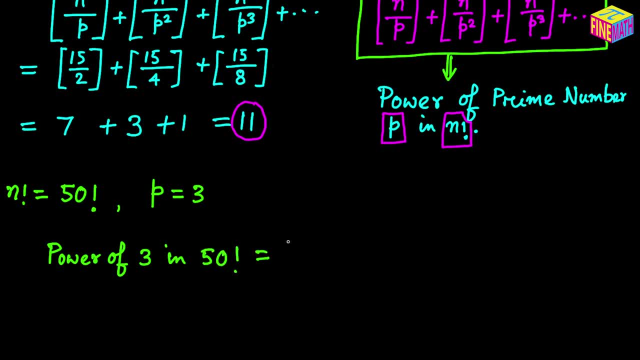 power of 3 in 50 factorial is equal to the greatest integer of the first one would be 50 divided by 3. and then we will do 50 divided by 3 square, greatest integer of 50 divided by 3 square. and then we will do again 50 divided by 3 cubed, and then again greatest integer.